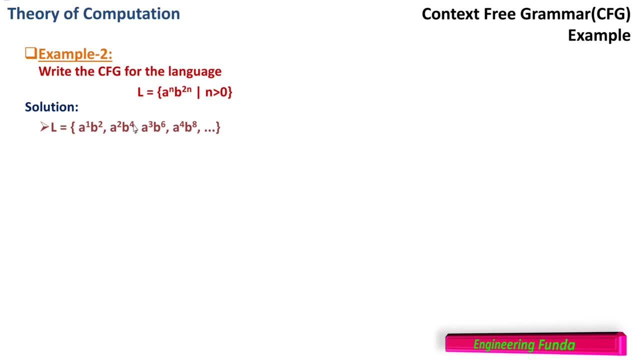 2 and b raised to 2 into 2, which is 4.. For n equal to 3, it will be a raised to 3, b raised to 6, and so on. Now, this we have already studied and we are aware that this power here indicates: 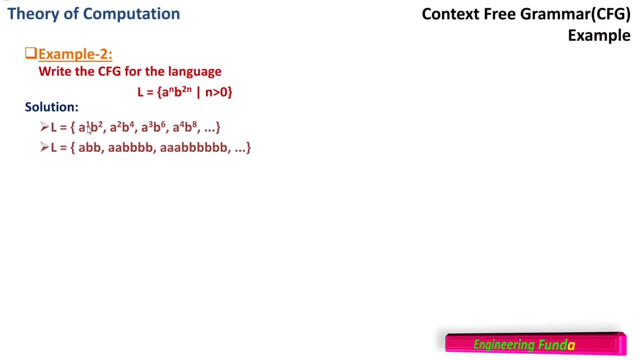 the number of occurrences. So my first word will have one occurrence of a and two occurrence of b. That means it will be a, b, b. For the second word, it is two occurrence of a and four occurrences of b. So it is a, a, b, b, b, b. That means we have two a's and four times b. Same way. 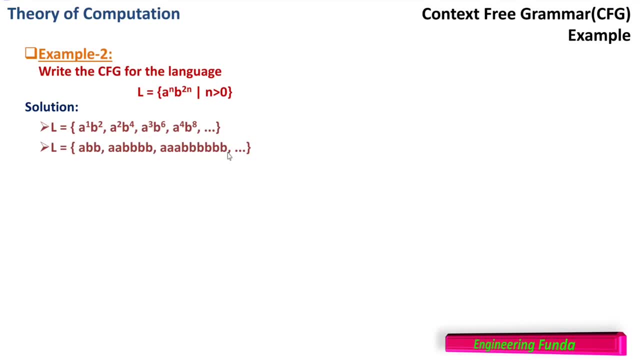 for a raised to 3,, b raised to 6, we will have triple a, triple b, triple b and so on. Here we will make use of the language L1, which is a raised to n. b raised to n, for n is greater. 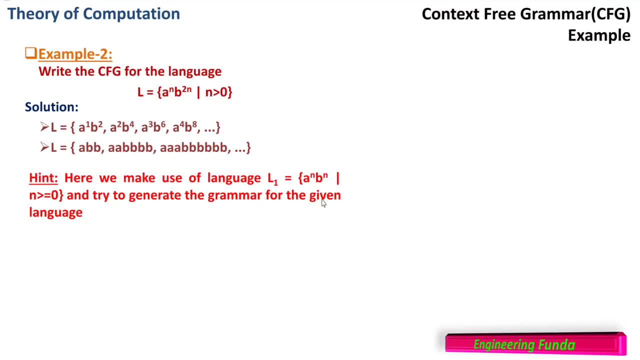 than equal to 0, and try to generate the grammar for the given language: a raised to n, b raised to 2n. But here we have to observe that the n value is greater than 0. It is not greater than or equal to 0. Hence the minimum word accepted here is a, b, b. That we can see. 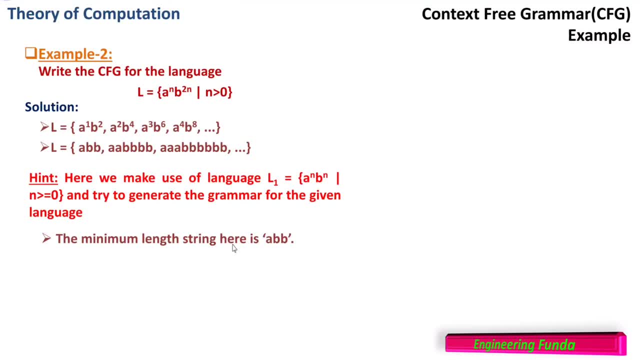 the first word is a, b, b. That is the minimum length string that is belonging to the language. So what we have to do is we have to add the production s tends to a b, b to the grammar for the language. 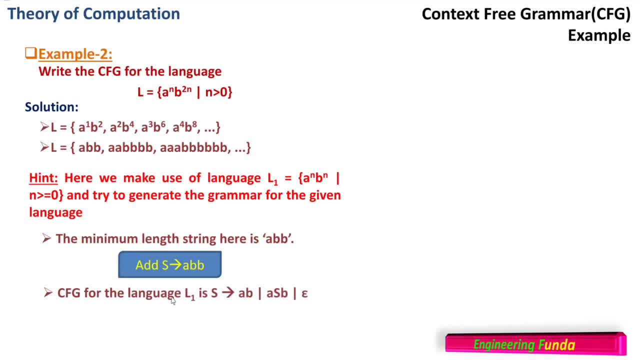 Now the context free grammar for the language L1, which is a raised to n, b raised to n, is s tends to a, b, or a s, b or epsilon. This we have seen just studied in the last part of this class, previous video. the language asked above does not accept epsilon because the 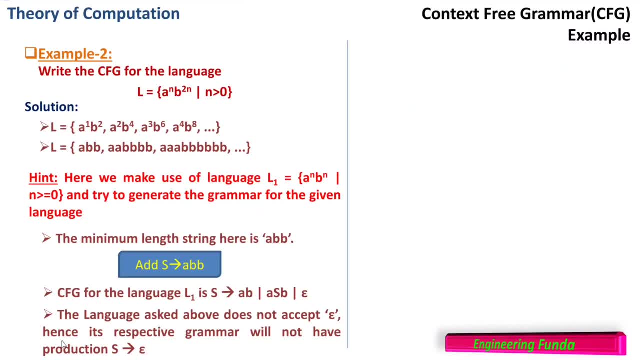 value of n is not equal to 0, hence its respective grammar will not have the production s tends to epsilon. so this is a key note that we need to remember: that if my null string is not accepted by the language, then the s tends to epsilon. that is the starting symbol tends to epsilon. production should not belong to. 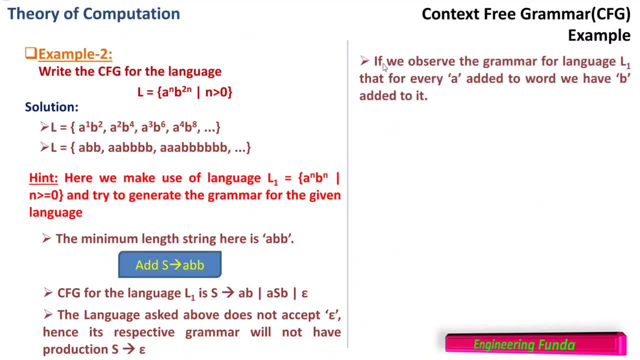 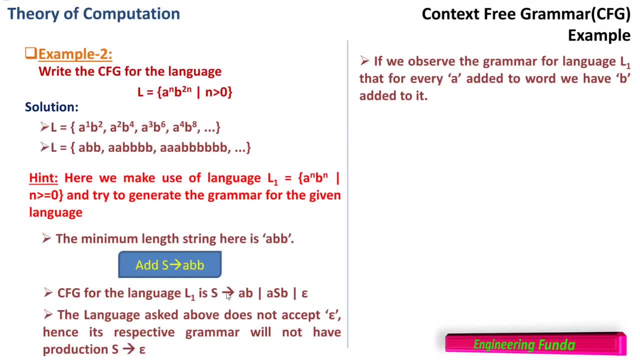 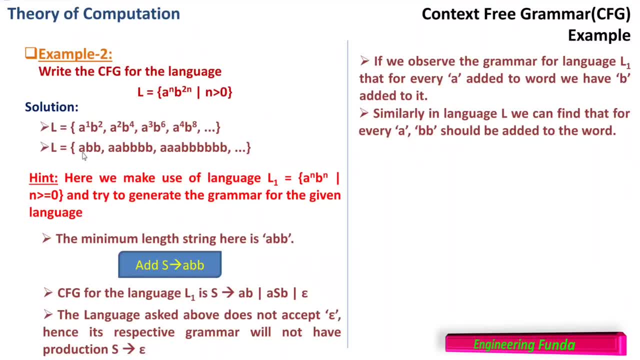 should be added to the word. so here for this one a, you have two B's. then for two a you have four B. that is a B, B and then a B B there. then triple a will have double B, double B, double B three times. so for each a there is a BB added to the word. now let us modify. 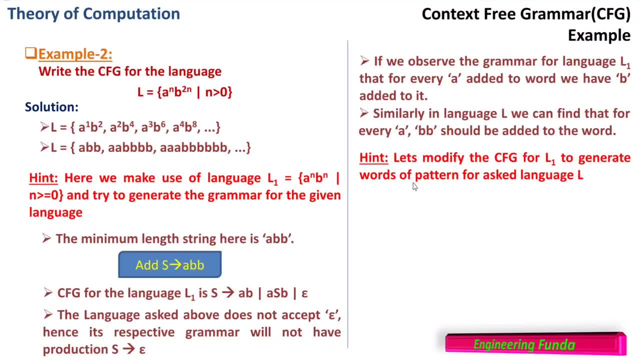 the context-free grammar for l1. to generate the words of pattern, ask for the language l. this is the context-free grammar for the language l 1, which is a raise to n, B raise to n in. it has three production rule: S tends to epsilon, S tends to a B and S tends to a s B, that we have two variation in each case: the. 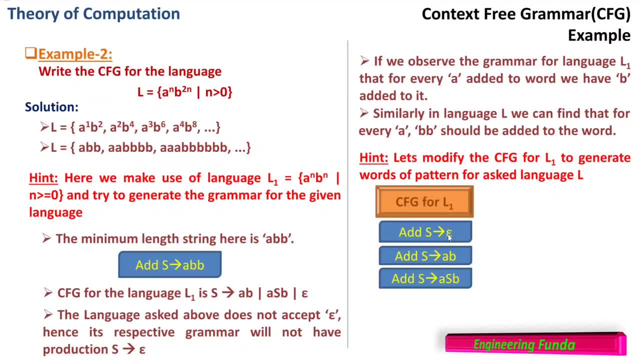 language has three formation rules for each one, so that once the words assume two b that we have seen Now the context free grammar for the language l, which is a raised to n, b raised to 2n, will have. so if we look at this, s tends to epsilon. we have just said that x, this null string. 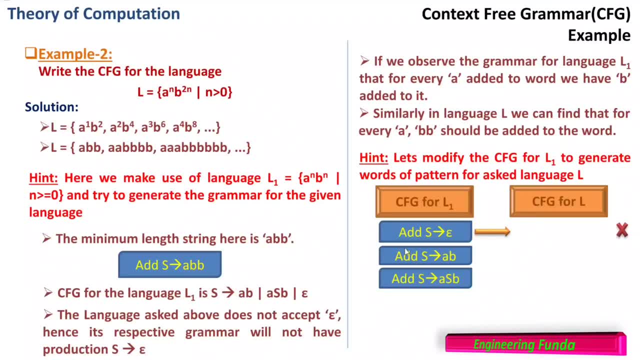 epsilon does not belong to the language, So this production will not belong to the language. context, free grammar for the given language. Then for s tends to ab. we know that for l1 there is a single a, and for every a you have a b. and then here you have an a and for every a you have a bb. 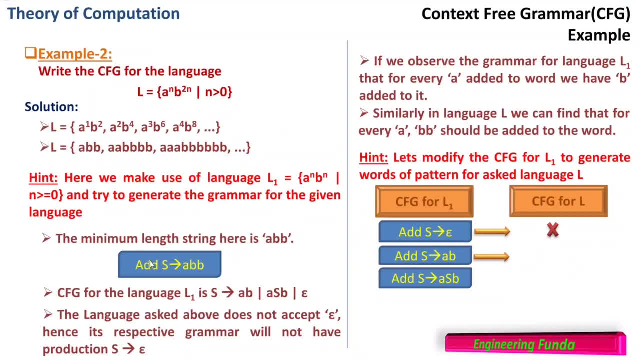 So my this production s tends to ab will become s, tends to ab, b. So we are adding this production s tends to ab To my context free grammar. In the same way, this production s tends to a is b, which is used for generating the subsequent words by adding a and b in the language l1.. So here what we will do is: 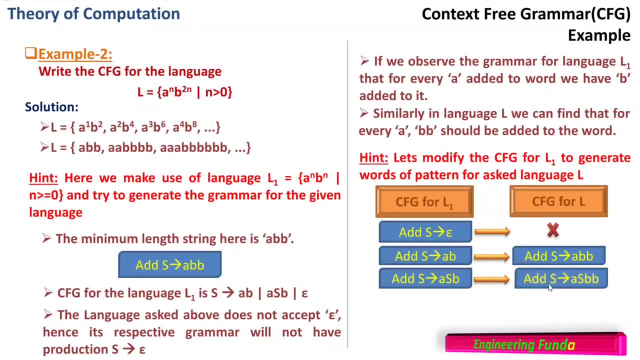 for every a you need to add a bb, So here my production will become s, tends to a, s, bb. So for every time you use this production, there is one a and two b added to the word. So if you want to generate this- a, a, bb, bb, this word, a raised to 2, b raised to 4- then we have to use this: 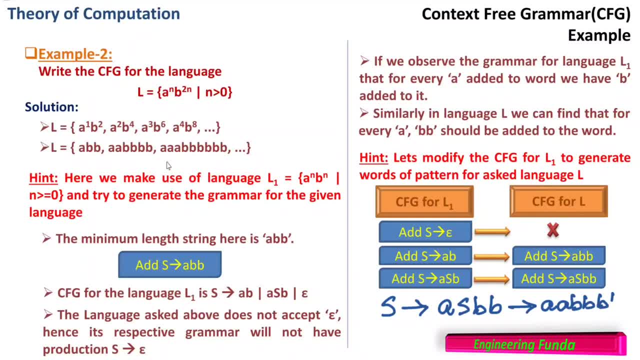 production once s tends to a s b, and then the innermost a bb can be generated by using s tends to a bb. Same way for a raised to 3, b raised to 6. that is this triple a, triple b. We have to use this production s tends to a s b, Then again a s b is replaced with. 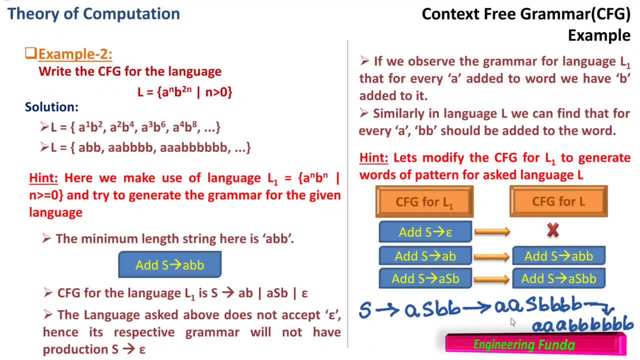 a s b. That means you will have now double a s, double b, double b, and then we will stop by using this production s tends to a bb to generate this: a raised to 3, b raised to 6.. Hence my, finally, the context free grammar for the language l is a raised to 3, b raised. 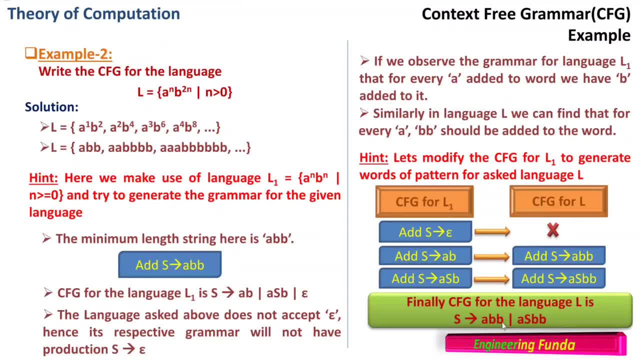 to 6.. Hence my, finally, the context free grammar for the language l is a raised to 3, b raised to 6.. So this is s tends to a bb, this production, and s tends to a s bb, that is a s bb. So this: 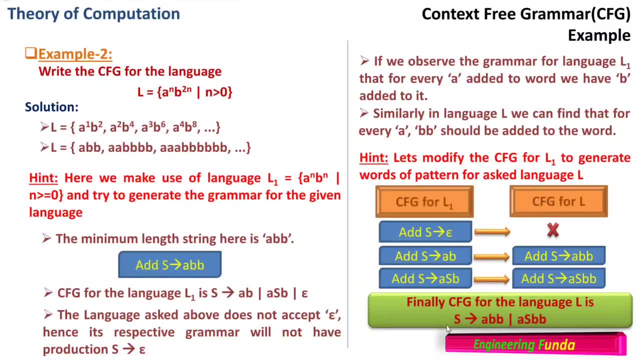 grammar s tends to a bb or s tends to a s bb is my context free grammar for the language l equal to a raised to n, b raised to 2n. I hope this approach of using a known grammar in generating the grammar for a new language 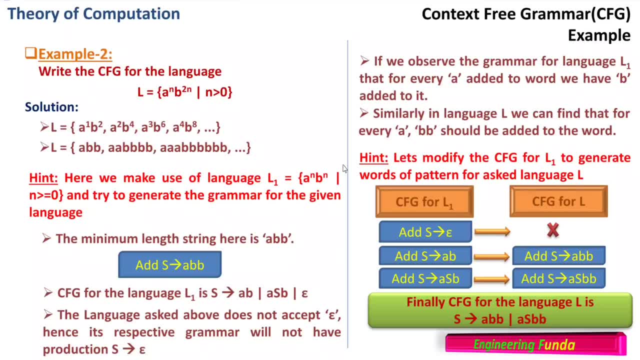 is understood very well and you can apply this approach to many given languages. thank you for watching this video. my dear friends, stay tuned for more videos on theory of computation lecture series.